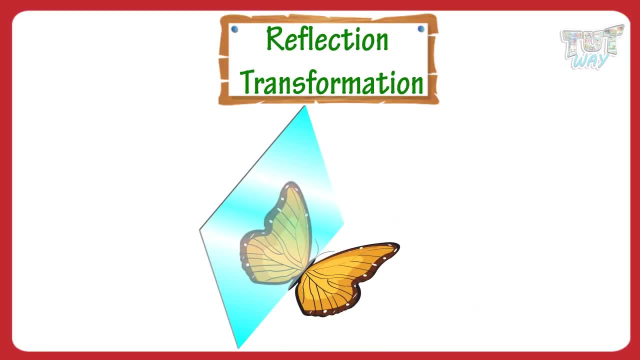 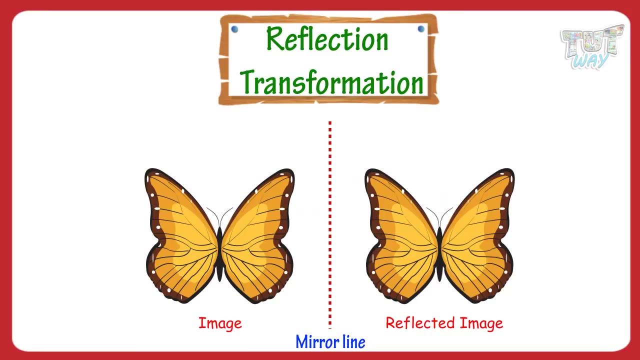 If you place a mirror on the line of symmetry of an object, you see the other half in its reflected image, And if you place mirror on any edge of a 2D figure, you will get its reflection. Here are more examples of reflected images. 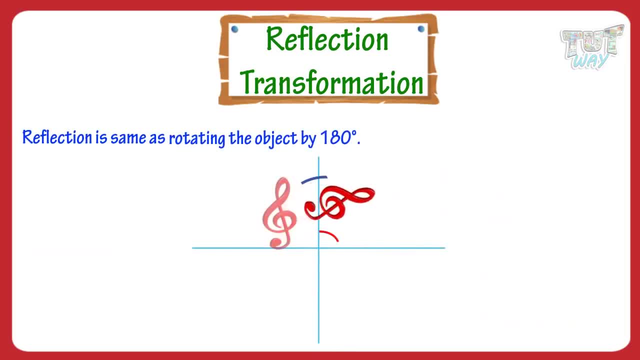 Reflection is also the same as rotating the object 180 degrees. like this, Points on an image and its reflection are equidistant from the line of reflection or mirror line. When a point is reflected, it is reflected in the mirror. When a point is reflected in a mirror line, the point and the image of the point are equidistant or same distance from the mirror line. 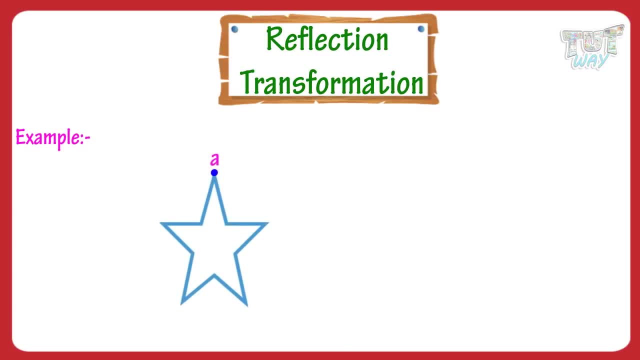 Let's have a look at example. A is the point on actual image and A' is the point on reflected image. Both the points are equidistant from the mirror line. Let's have a look at another example. A'B'C is a reflected triangle. then 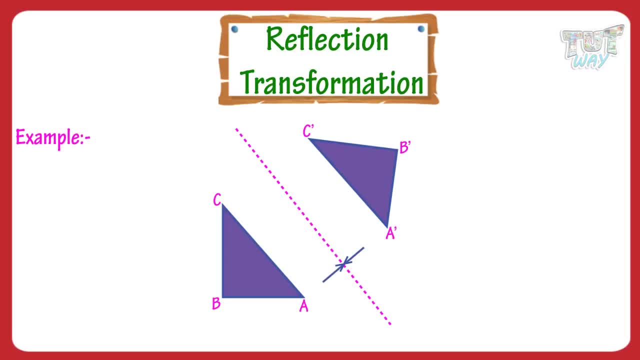 A and A' are equidistant from the line of reflection. B and B' are equidistant from the line of reflection. C and C' are equidistant from the line of reflection. A figure and its reflected image are always congruent to each other. 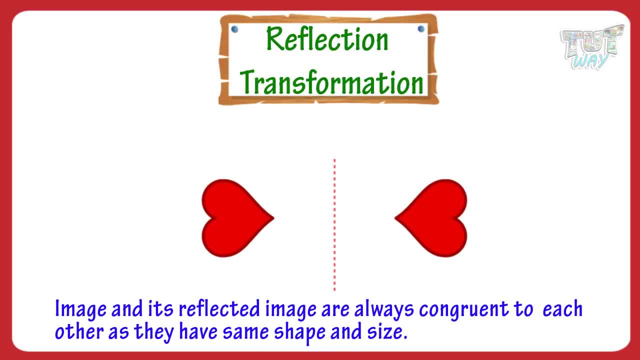 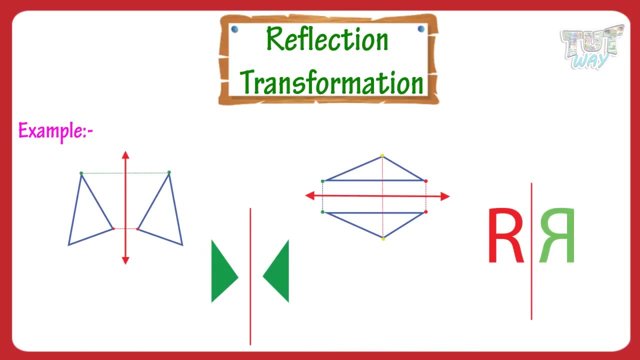 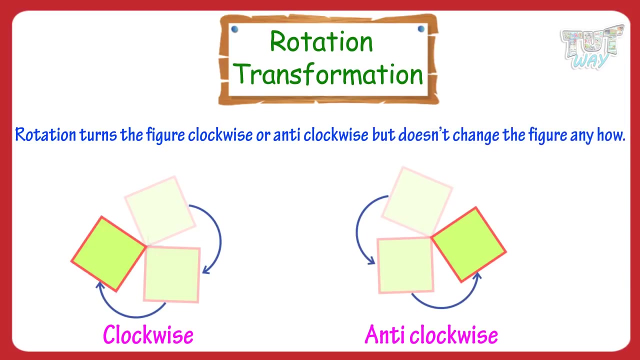 That is, they have same shape as well as same size. A figure and its reflected image are congruent, but face in opposite directions. Here are examples. Now let's learn another type of transformation. It is rotation. Rotation turns the figure clockwise or anticlockwise, but doesn't change the figure anyhow. 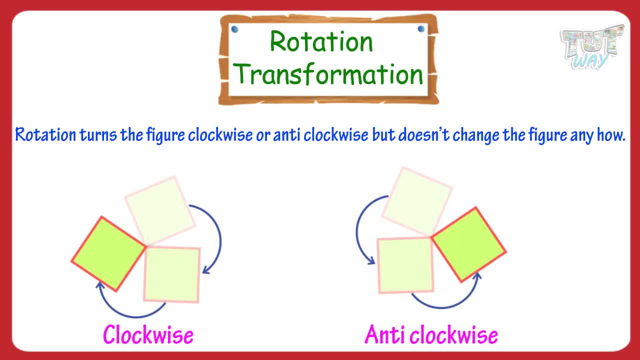 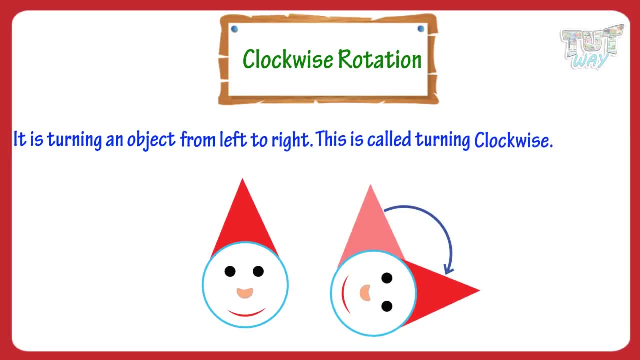 That is, shape and size of the image are not changed. It is turning an object from left to right. It is called turning clockwise. Let's have a look at some examples. This is image A after transformation of 90 degree clockwise turn or rotation. 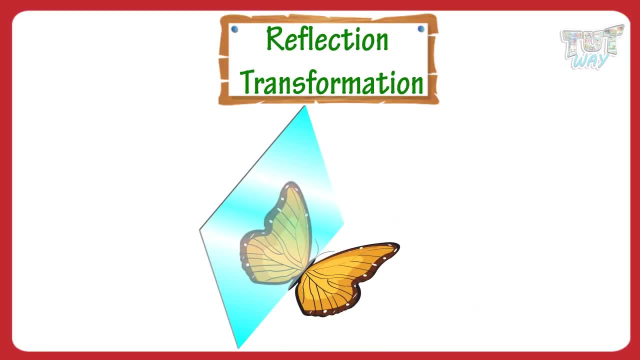 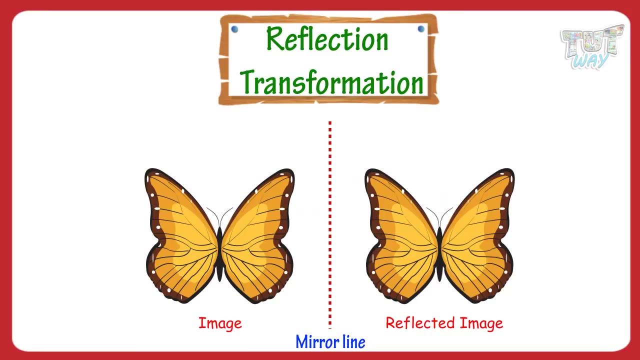 If you place a mirror on the line of symmetry of an object, you see the other half in its reflected image, And if you place mirror on any edge of a 2D figure, you will get its reflection. Here are more examples of reflected images. 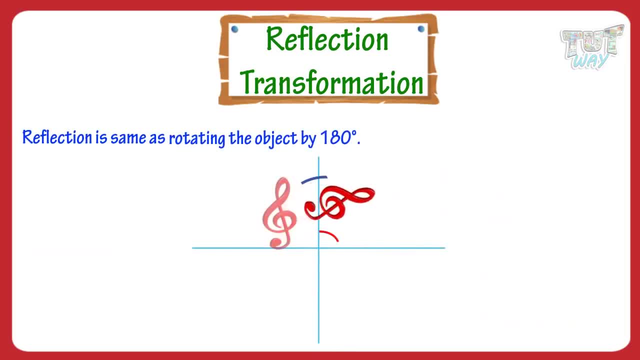 Reflection is also the same as rotating the object 180 degrees. like this, Points on an image and its reflection are equidistant from the line of reflection or mirror line. When a point is reflected, it is reflected in the mirror. When a point is reflected in a mirror line, the point and the image of the point are equidistant or same distance from the mirror line. 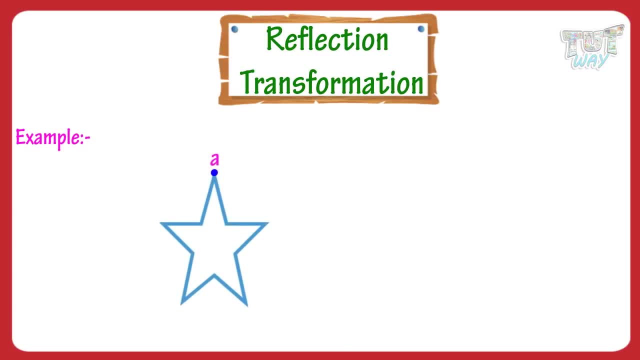 Let's have a look at example. A is the point on actual image and A' is the point on reflected image. Both the points are equidistant from the mirror line. Let's have a look at another example. A'B'C is a reflected triangle. then 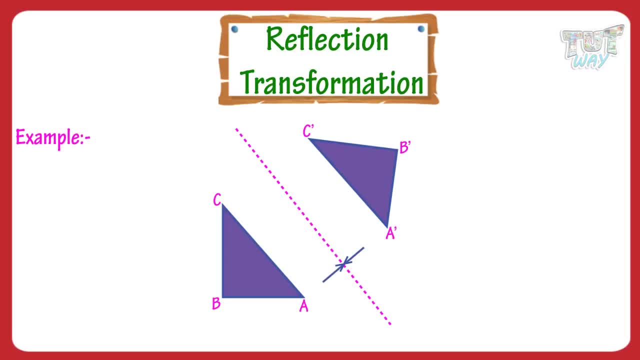 A and A' are equidistant from the line of reflection. B and B' are equidistant from the line of reflection. C and C' are equidistant from the line of reflection. A figure and its reflected image are always congruent to each other. 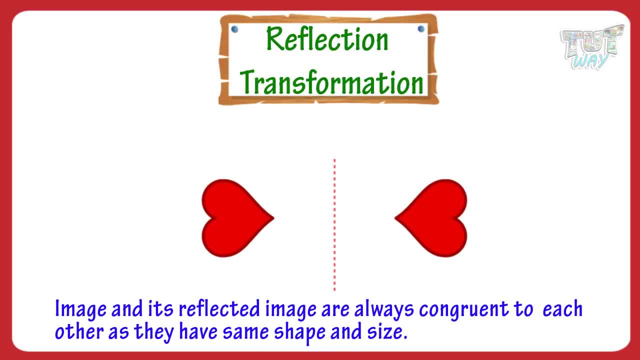 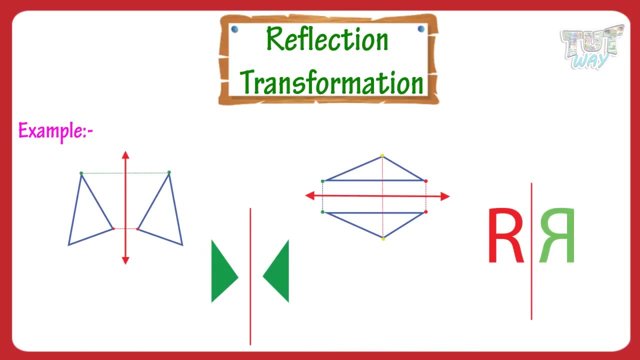 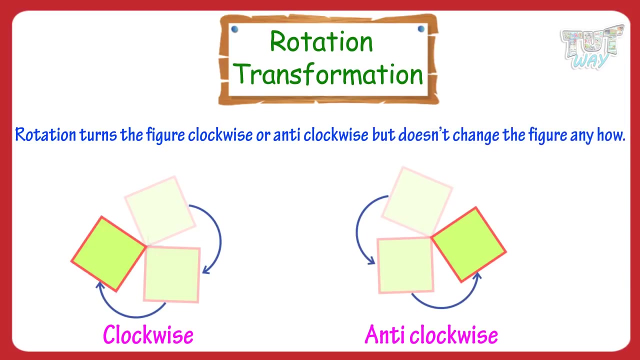 That is, they have same shape as well as same size. A figure and its reflected image are congruent, but face in opposite directions. Here are examples. Now let's learn another type of transformation. It is rotation. Rotation turns the figure clockwise or anticlockwise, but doesn't change the figure anyhow. 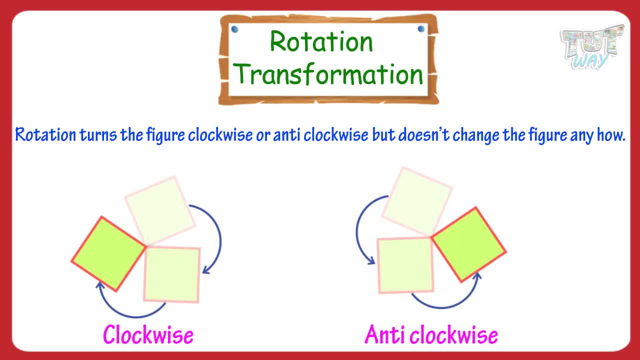 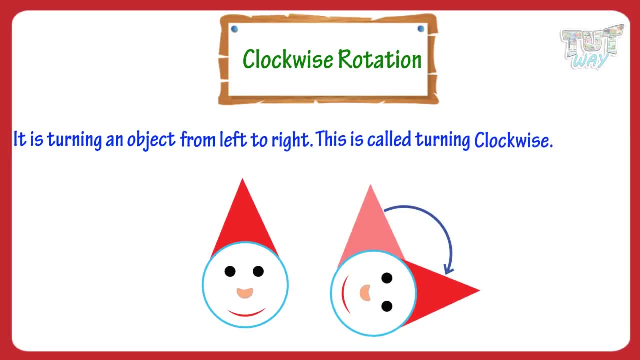 That is, shape and size of the image are not changed. It is turning an object from left to right. It is called turning clockwise. Let's have a look at some examples. This is image A after transformation of 90 degree clockwise turn or rotation.